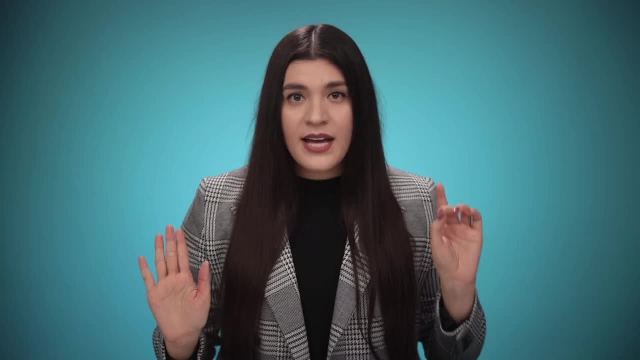 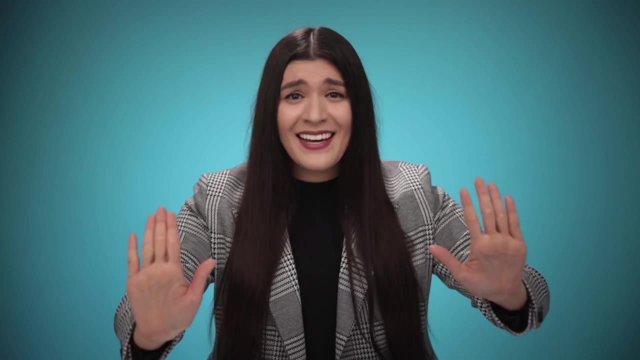 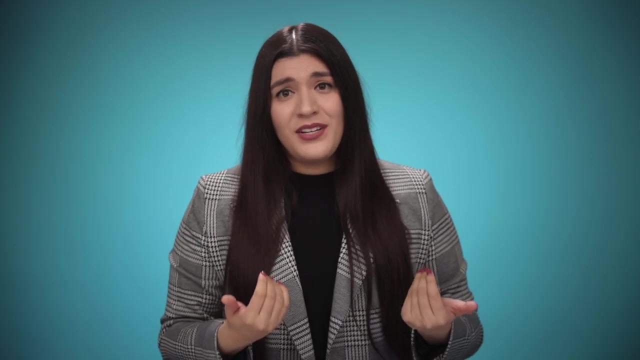 to the first video. I know some things may feel tempting to skip because they seem a bit easy at first, but please, please, please, don't skip anything. This playlist is already in the best order for you to really improve your math skills and avoid making common mistakes. I believe in you. 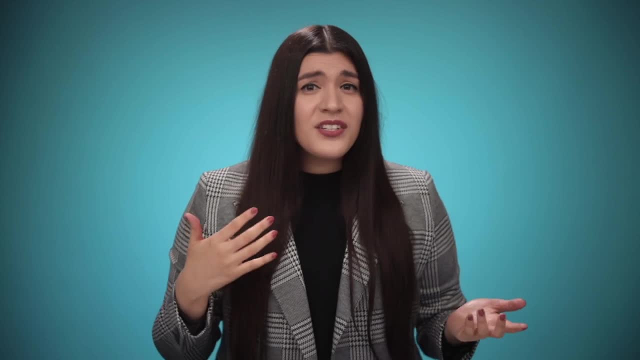 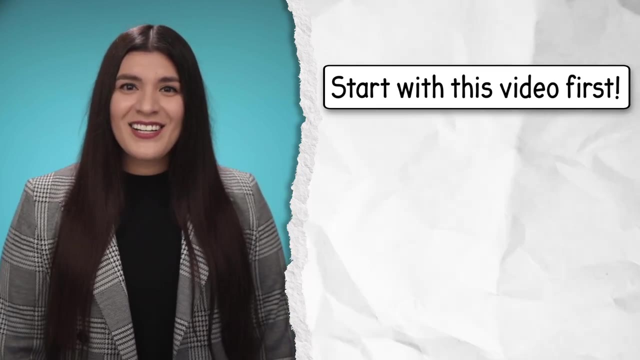 and know you are capable of understanding this. It's just going to take some time and effort, but you and me are in this together, So click the next video and let's get started. 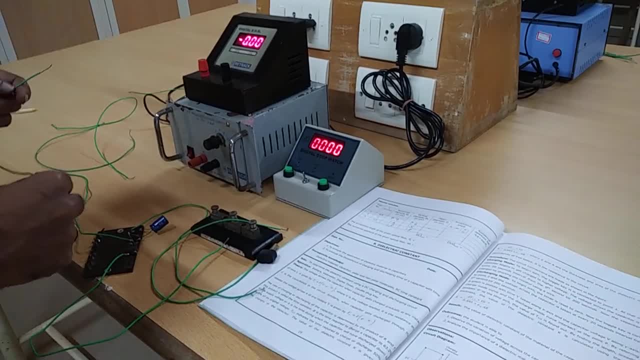 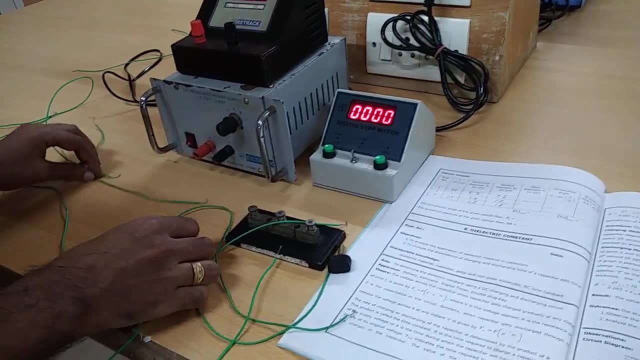 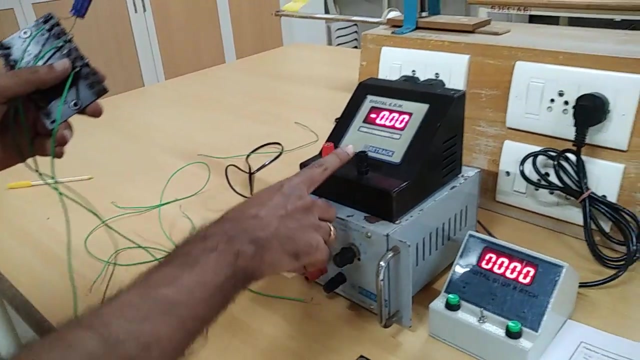 Dear students, so in this presentation I am going to discuss about dielectric constant experiment. So here the aim of the experiment is to find out the dielectric constant of the material which is used inside the capacitor. So this is a capacitor and here there is a resistor and we have a voltmeter, here a battery, a key and a digital stopwatch. 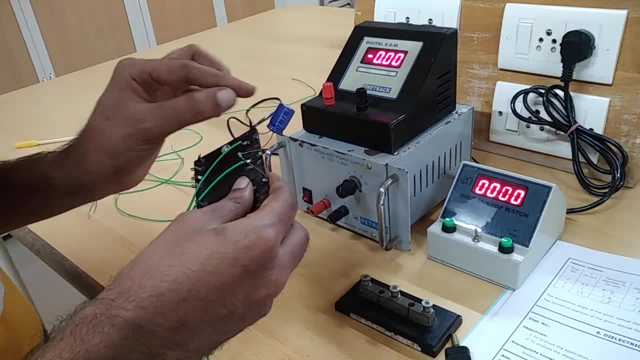 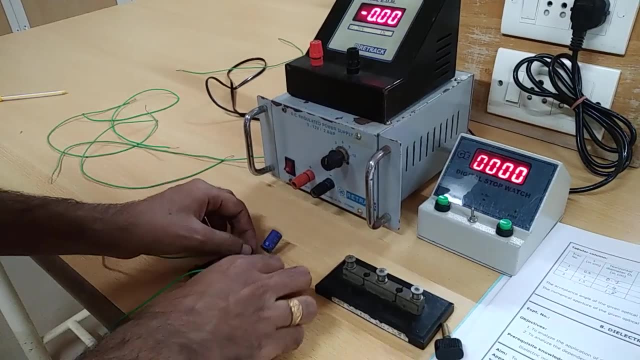 So what we do in this experiment is we are going to find out the voltage across the capacitor as a function of time. So let me do the connections first. See, this is the negative of the capacitor. there is a mark over here, white mark, and this is the positive. 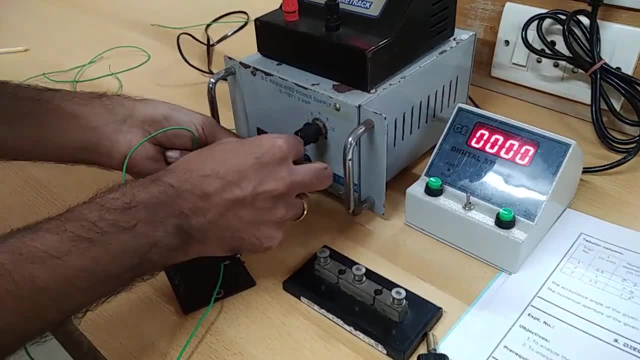 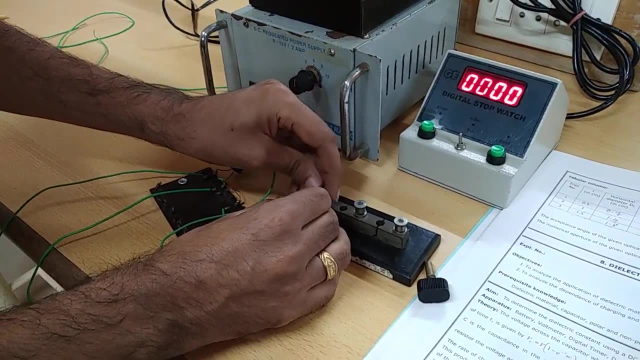 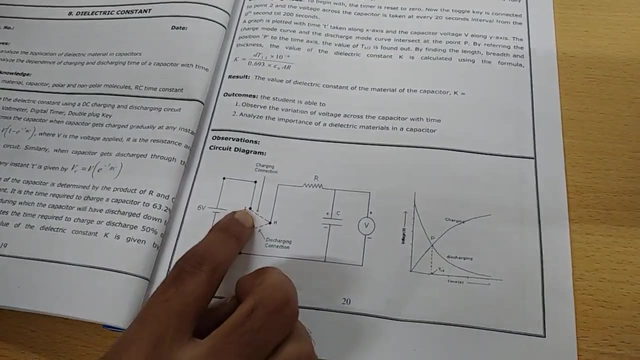 So from the battery, positive, see, it is given to one end of the key, so like this. And the negative of the battery And is given to. so if you look at this, the positive is given to one end of the key, negative is given to the opposite end. 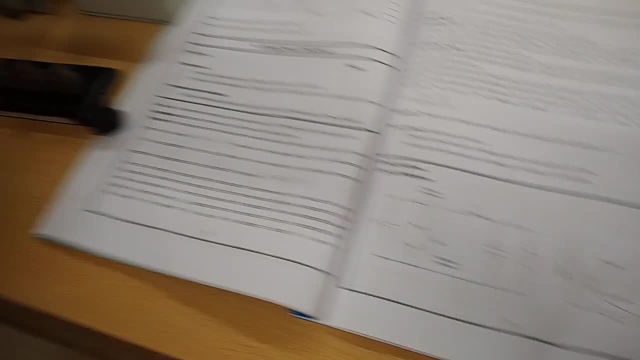 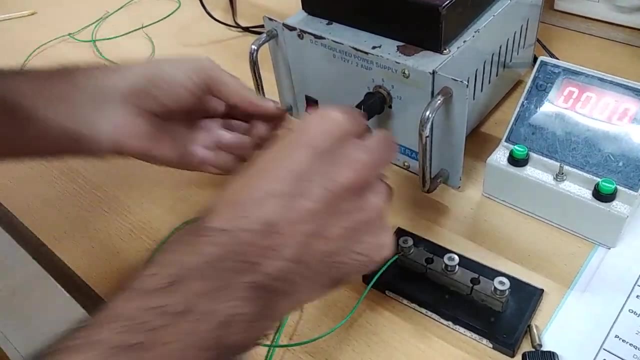 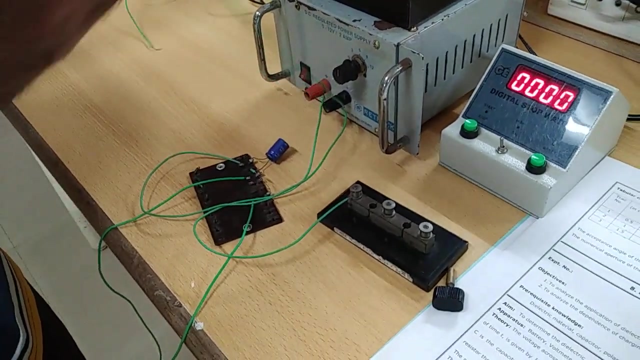 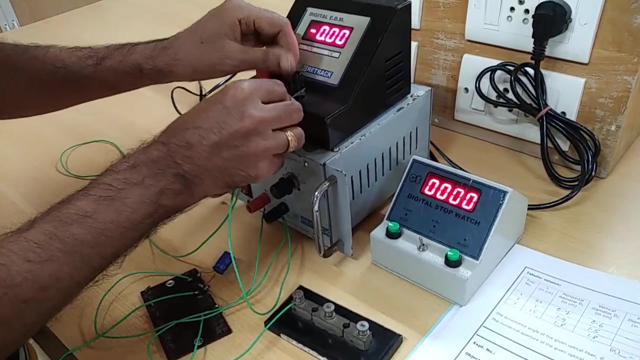 From the same point, one to the capacitor negative and voltmeter negative. So take a wire, capacitor negative, So just give to the battery: negative, And one more to voltmeter negative. One more, One more wire, so here voltmeter negative. and from the same point it is given to the opposite end of the key. so that is here.